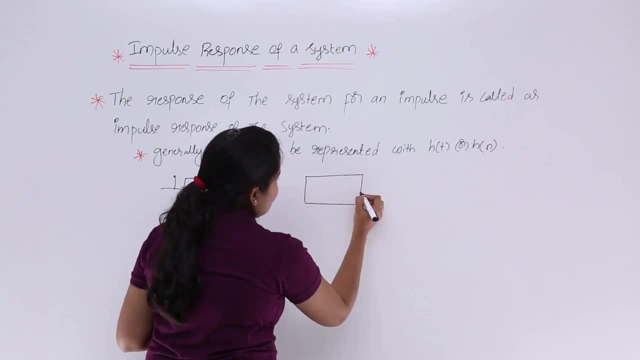 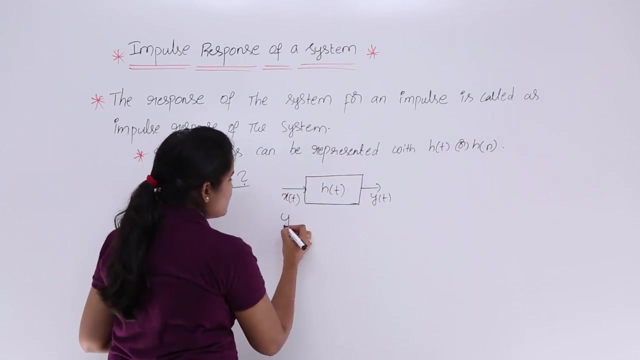 here we are having any system with impulse response H of T and input X of T and we are considering output as Y of T means. here if you want to write the relation between input, output and impulse response, that can be reduced, written as output of a system. always output of a system is equivalent to, So generally 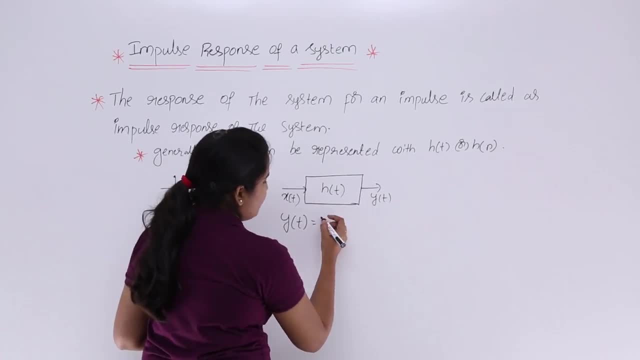 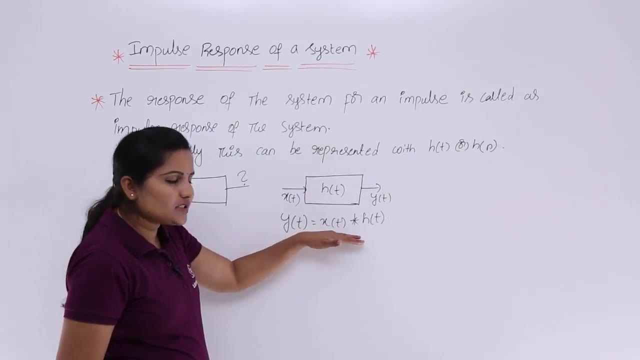 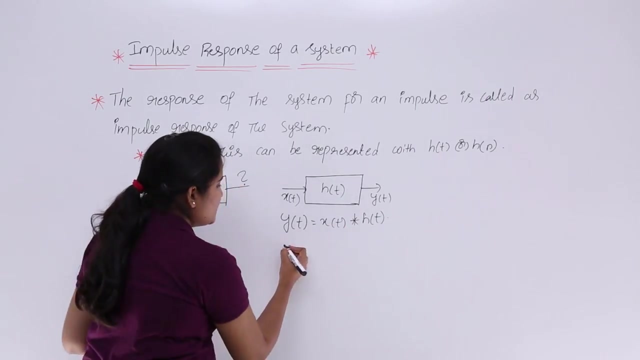 we will consider LTI systems. So output of a system is equivalent to input convolution with impulse response Here. this is time domain. if you want to write in frequency domain then you can have multiplication here. that means in frequency domain. h of s are that means? 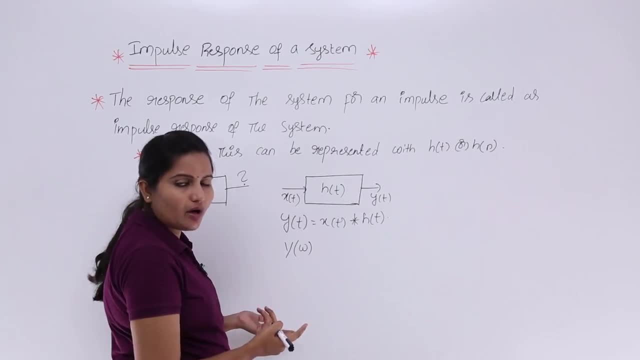 in omega or s. that means Laplace transform or Fourier transform. you can take any transform to get the frequency domain. I am considering Fourier transform here. that is why I have written omega. if you are considering Laplace transform, then you can write s here, So y. 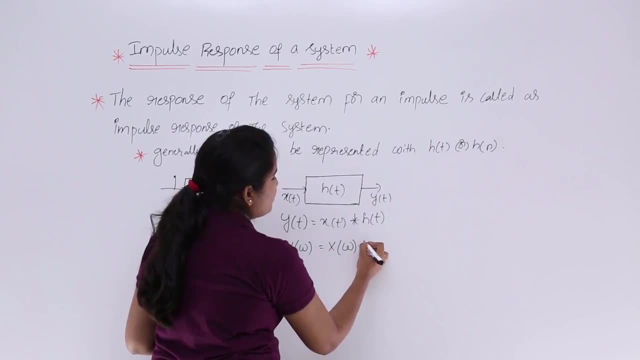 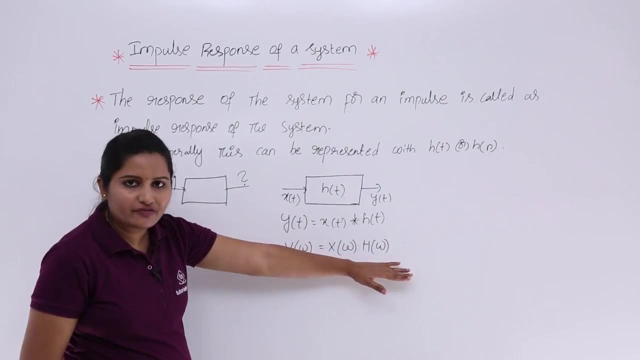 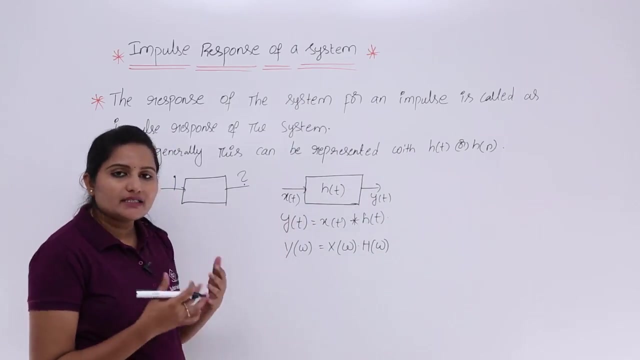 of omega is equivalent to x of omega into h of omega. So now here, if you want to calculate your h of t, that means from this equation. if you want to calculate your h of t, that calculate impulse response again, for example, in exams they will provide like this for a signal: 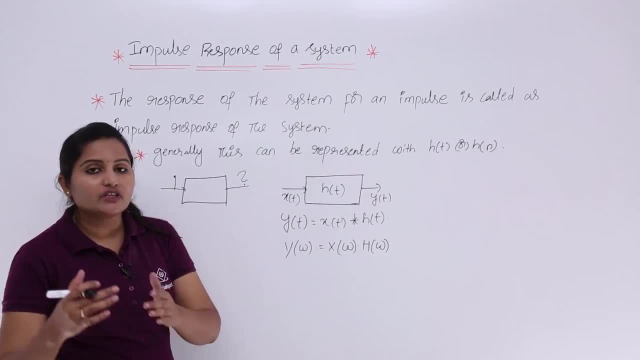 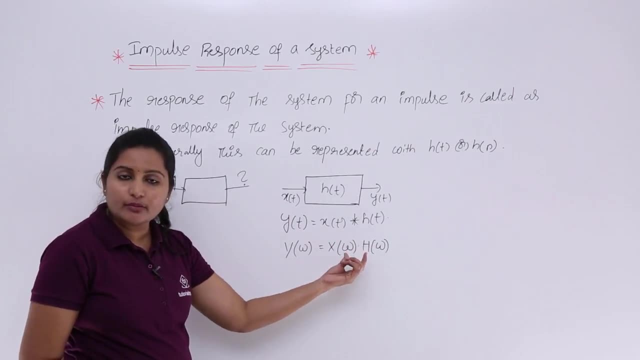 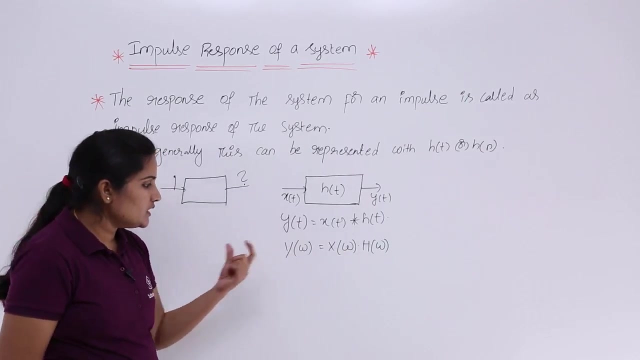 with, for a signal is given to a system with a response so and so what may be the impulse response of the system? they will ask like this: so they will provide both input and output, but they will ask impulse response. so by that we know the relation between these three. so here, by this, 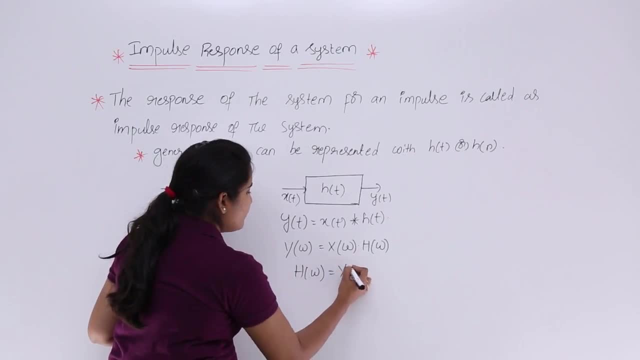 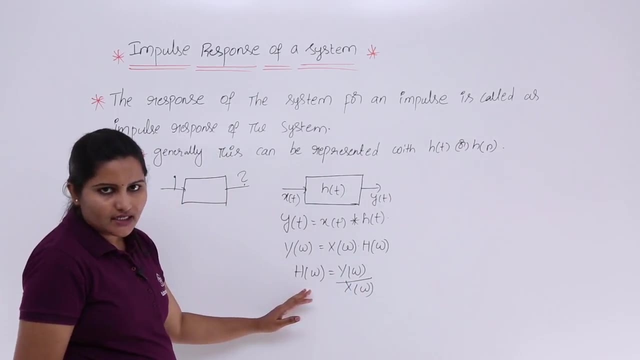 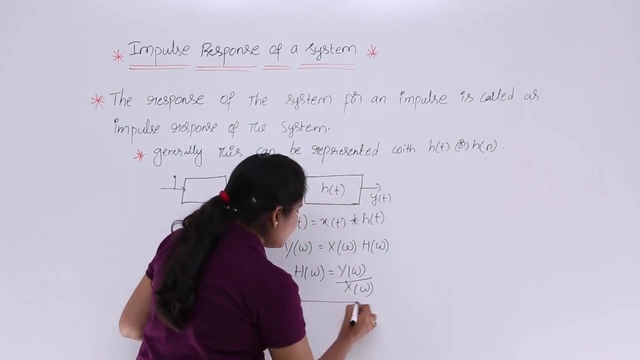 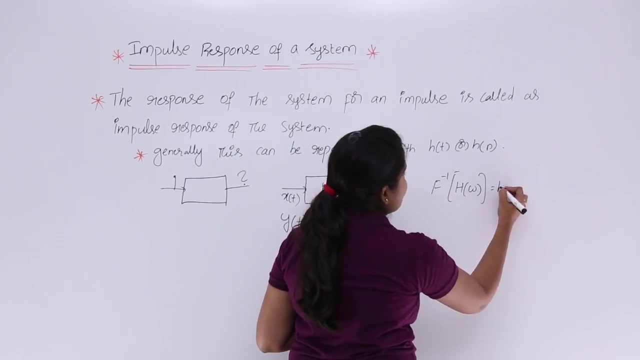 we can say: h of omega is equal into y of omega by x of omega. so if you consider inverse Fourier transform here, then you are going to get so h of t. so that means, after calculating h of omega, if you consider inverse Fourier transform of h of omega, you are going to get h of t. that means 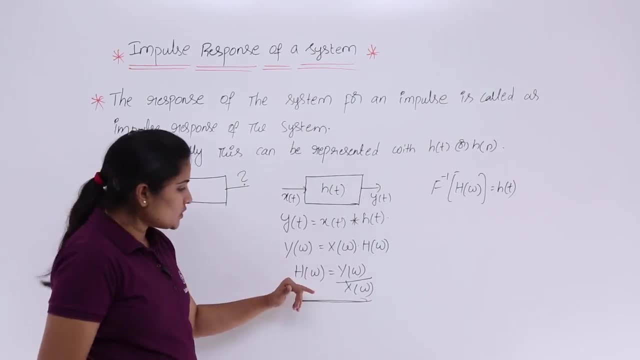 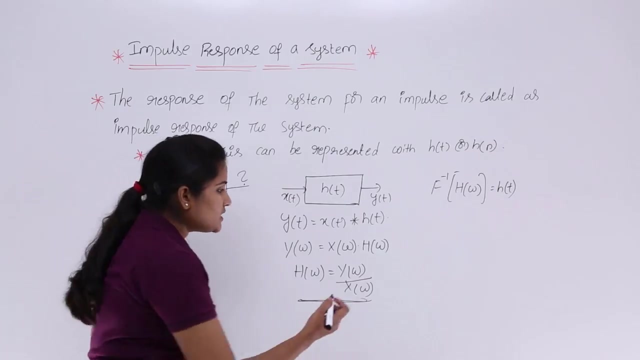 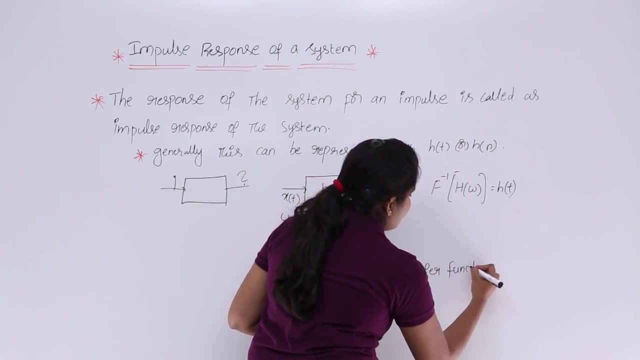 impulse response. so here, if you observe, so h of omega is there. this is always called as transfer function of a system. so here impulse response, transfer function are related. the transform of impulse response is nothing but transfer function, which is the ratio of output transform by input transform. so this is transfer, transfer function of a system. 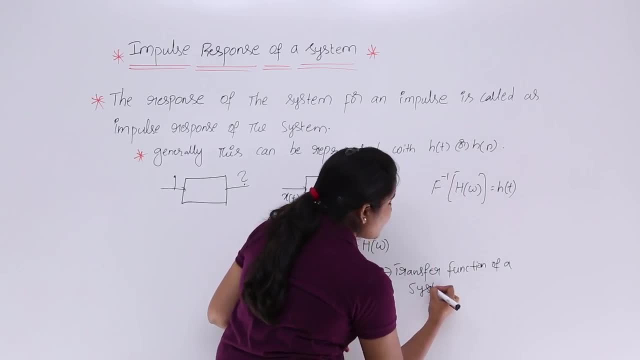 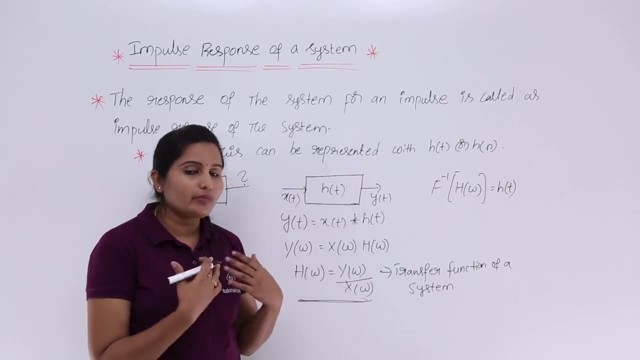 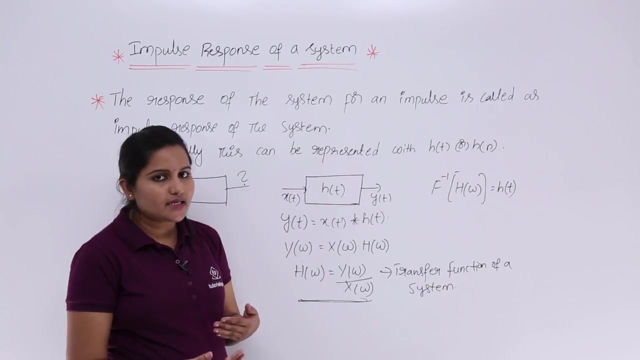 transfer function of a system. for example, in any exam they given like this: a transfer function of a system is given, then what may be its impulse response? they are asking like that. so you know the relation between transfer function and impulse response. if they given this to get impulse response, you need to consider. 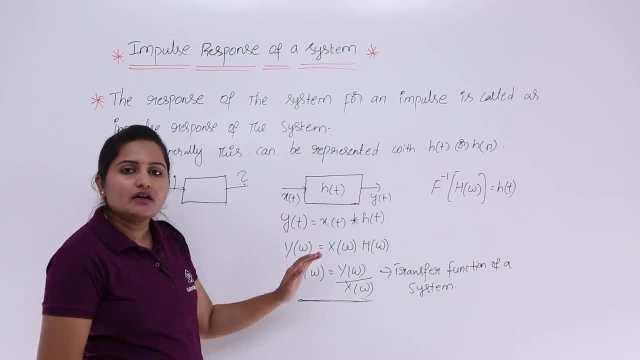 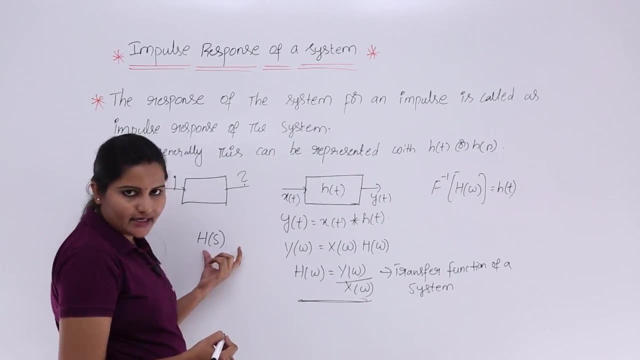 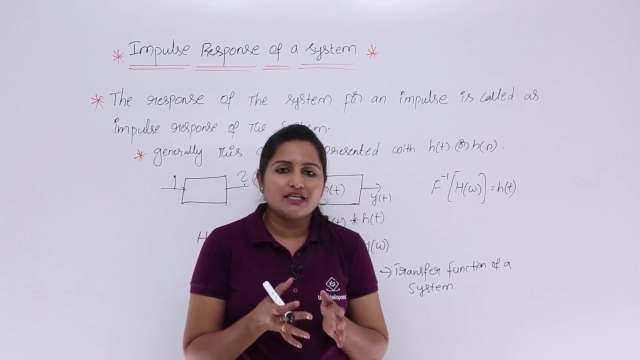 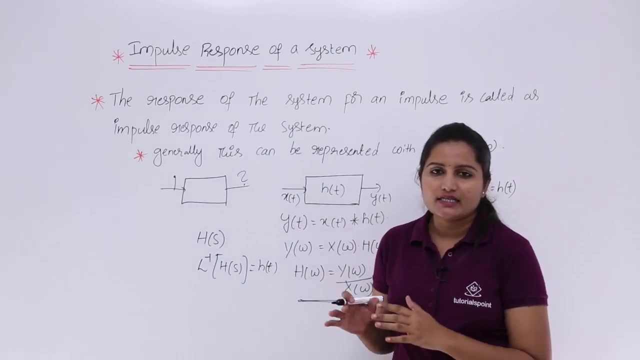 inverse transform. for example, if they given in a Laplace domain, that means s domain. for example, if they given transfer function of a system, then what may be its impulse response? that means h of s. if you want to consider impulse response from this, then inverse Laplace transform you need to consider h of s is equivalent to h of t. inverse Laplace transform of h of s will provide h of t. or inverse Fourier transform of h of omega also going to provide h of t. so like this way you are going to deal the problems, so you can consider this topic under transfer function also: impulse response and transfer function of a system like h of s. if you want to consider impulse response from this, then inverse Laplace transform you need to consider h of s is equivalent to h of t. inverse Laplace transform of h of s will provide h of t. or inverse Fourier transform of h of omega also going to provide h of t. so like this way you are going to deal the problems, so you can consider this topic under transfer function also: impulse response and transfer function of a system like h of s. if you want to consider impulse response from this, then inverse Laplace transform you need to consider h of s is equivalent to h of t. inverse Laplace transform of h of s will provide h of t or inverse Fourier transform. 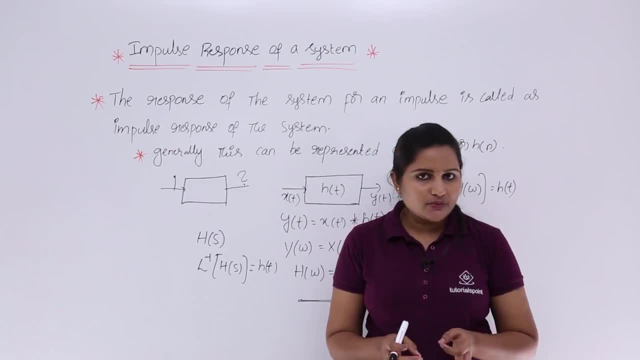 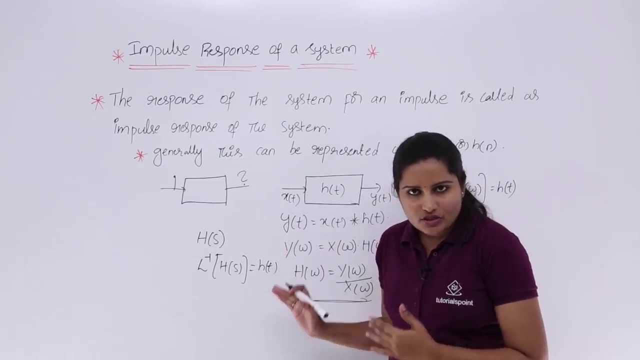 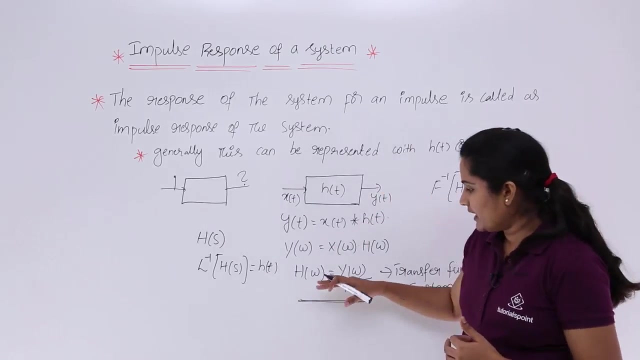 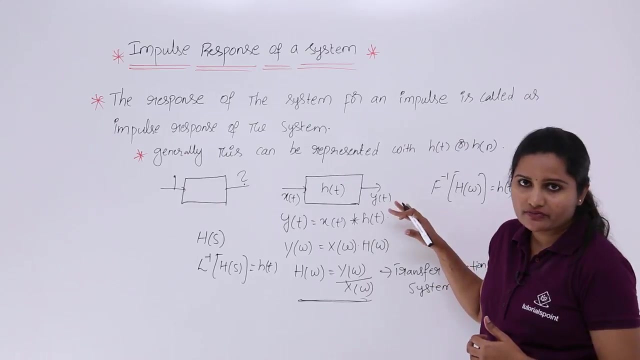 so impulse response is nothing. but this is the response came by giving input impulse as input. so coming to this transfer function, transfer function is the Fourier or Laplace transform of impulse function. this can be taken as output transform, by input transform. both are very important when you are calculating any response of this system. coming to the relation of input, output and impulse response, y of t is equivalent to h of s is equivalent to h of t. 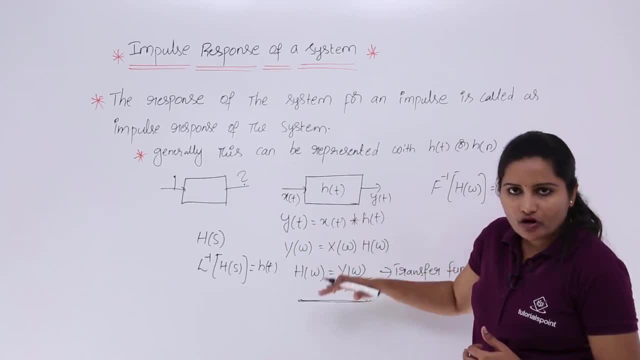 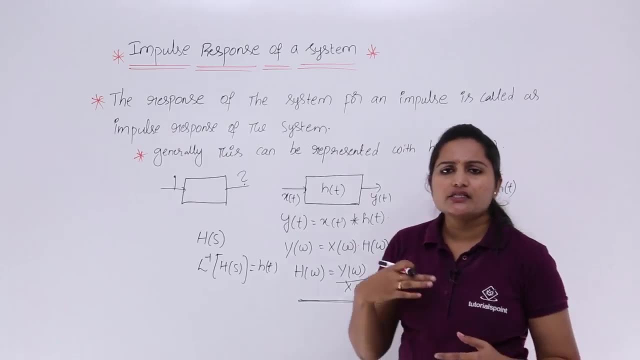 equivalent to x of t convolution with h of t. if you want to write in frequency domain and transfer function, then you can write in multiplication. so by these relations you can solve any question related to impulse response or transfer function or transforms.